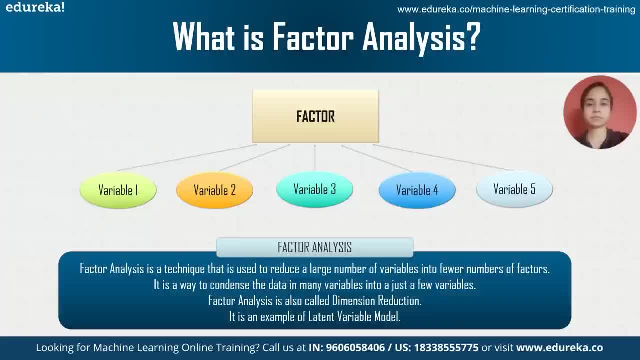 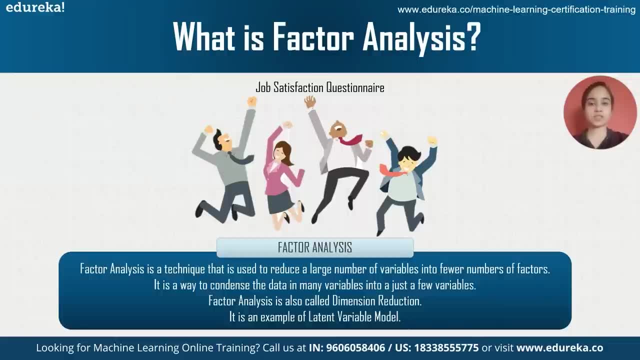 reduction, since it reduces the dimension or the total number of variables in the data set. Factor analysis is a kind of latent variable model. More on that later. Consider a job satisfaction questionnaire. As for a person's qualification supervisor, which can in turn depend on appraisal or 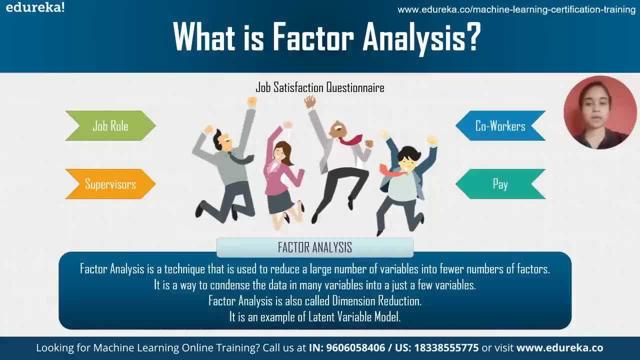 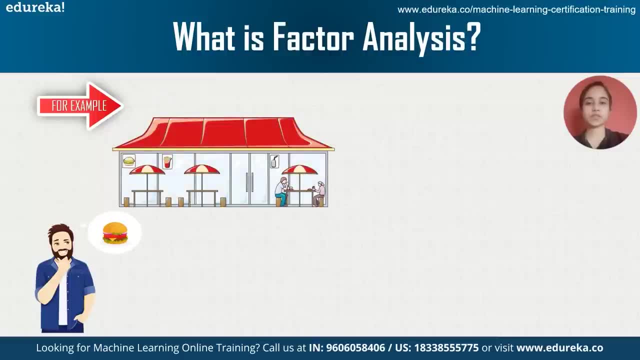 communication, satisfaction with co-workers, pay, etc. Let's take an example of factor analysis. Say that you are a foodie and you want to pick a restaurant to go to. So you start checking reviews on different restaurants. You find that the reviews are categorized on the aspect of six. 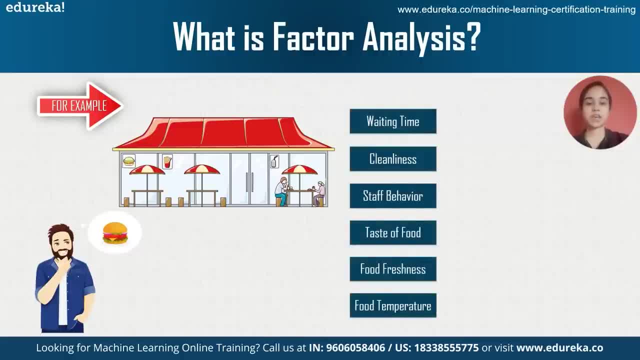 variables, which are waiting time, cleanliness, staff behavior, taste of food, food freshness and food temperature. Too many variables are making it difficult for you to pick a particular restaurant that you would go to The two factors to pick a restaurant that you really care about. 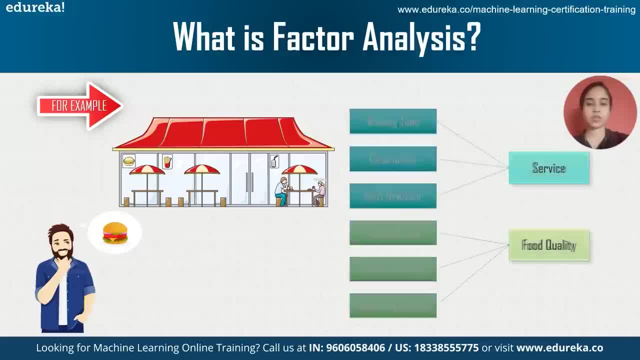 are, let's say, service and food quality. The variables in the reviews can be broadly categorized in these two factors, as shown. This is what factor analysis does. So service and food quality are not really present in the data, but are derived out of the data. These are called the latent. 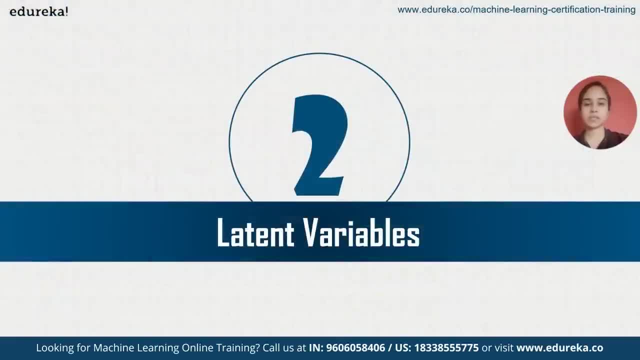 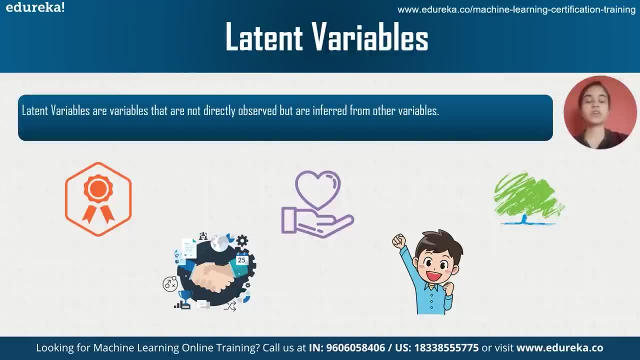 variables. Now let's have a deeper dive into what latent variables are. In statistics, latent variables are variables that are not directly observed, but are rather inferred from other variables that are observed. This is what we call factors. It's actually difficult to measure numerically The mathematical model that aims to explain observed variables in 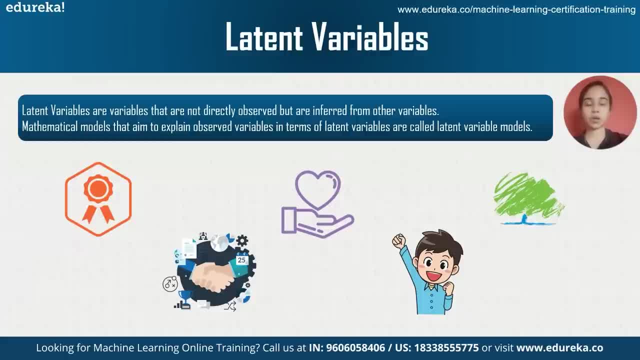 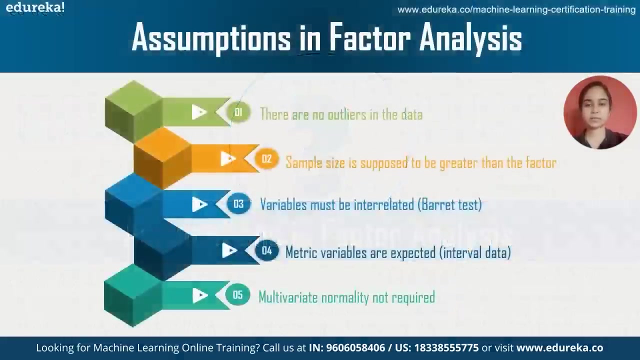 terms of latent variables are called latent variable models. Hence, factor analysis is a latent variable model. Examples of latent variables are quality of life, business confidence, morale, happiness and conservatism, among others. Now, in order to perform factor analysis, certain assumptions are made about the data. Let's have a look at these. Firstly, 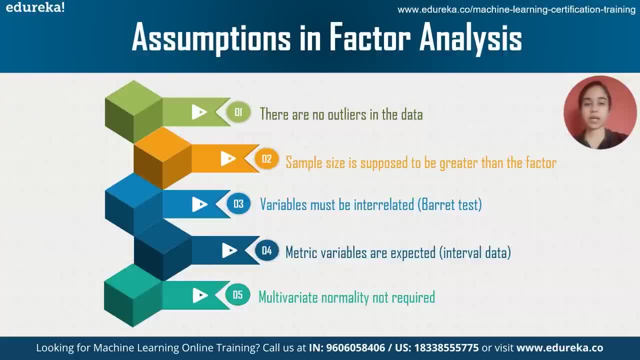 we assume that our data is clean. There should be no outliers or missing values. Secondly, the sample size is expected to be greater than the number of factors. A general principle is the minimum 1 to 5 ratio, That is for, let's say, 10 factors. 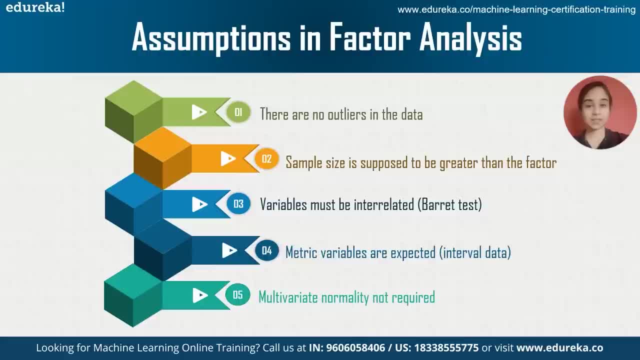 you should have around 50 samples at least. Thirdly, the variables are expected to be interrelated. The concept of factor analysis is based on correlation of data so that it can be grouped together. We can perform something called Barrett test to analyze the correlation. 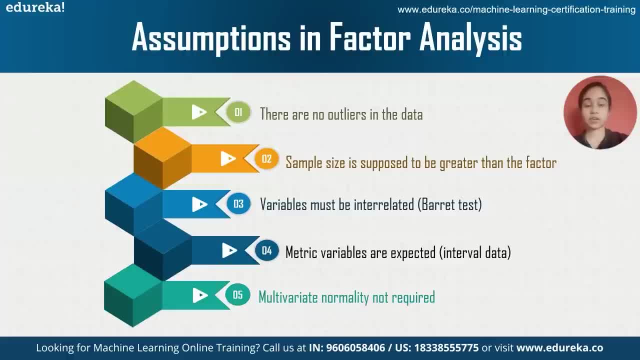 Next, matrix variables are expected, That is, the variables are expected to be of numeric type, It should be in an interval of numbers And, lastly, the data is preferred to be normalized. However, multivariate normalization is not necessary Now. 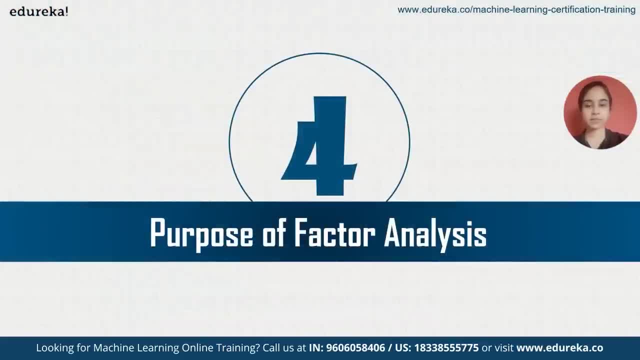 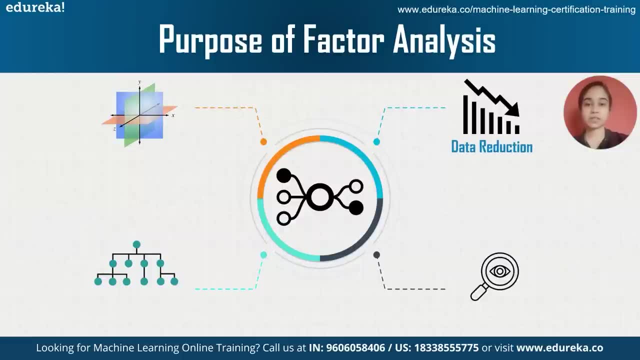 let's have a look at the purpose of using factor analysis. The primary purpose of using factor analysis is for data reduction. Having too many related fields can make it difficult to analyze the data. Thus, factor analysis reduces the number of variables. It also helps in latent variable discovery, as we saw in the examples before. Some factors: 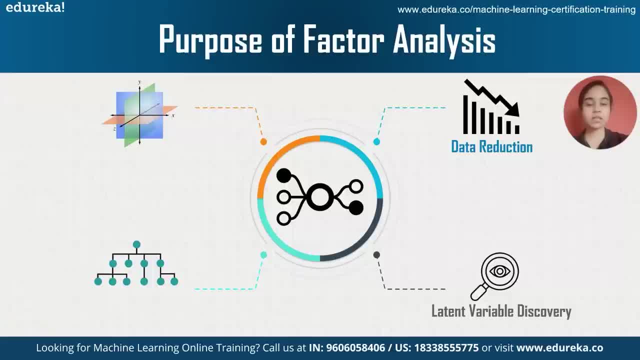 such as empathy, cannot be measured, but it can be formulated using other variables. Factor analysis supports simplification of items into subset of concepts. Sometimes, many fields in our data signify the same thing, Such as in the restaurant example. delay in serving staff, behavior and cleanliness signify the same factor, which is service. Moreover, with 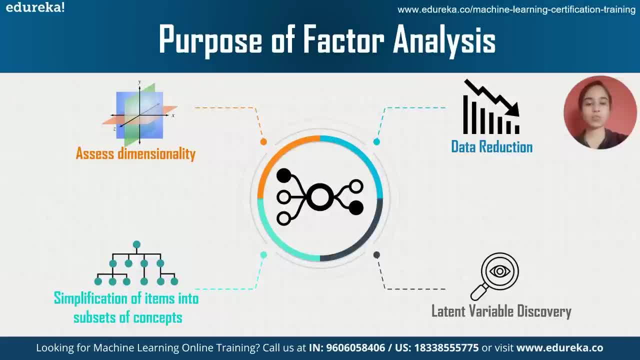 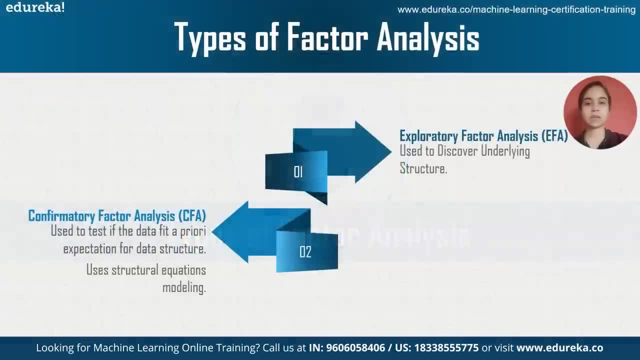 factor analysis. you can access the dimensionality and homogeneity in the data. Now let's move on to the types of factor analysis. Factor analysis can be broadly classified into two types: EFA and CFA. Exploratory factor analysis is used to 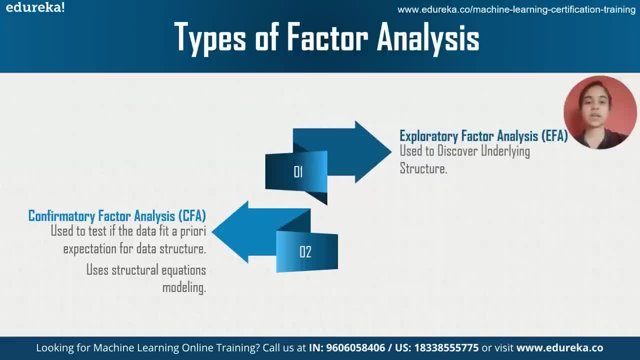 discover the underlying structure in the data using something like correlation matrix. It is used for getting insights out of the data And confirmatory factor analysis is based on the correlation matrix derived in EFA. So CFA is used to test those expectations It makes use of. 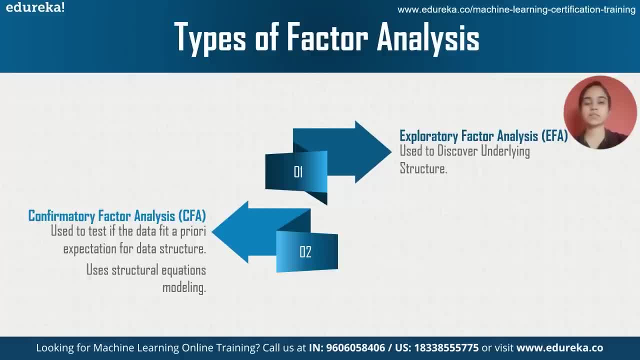 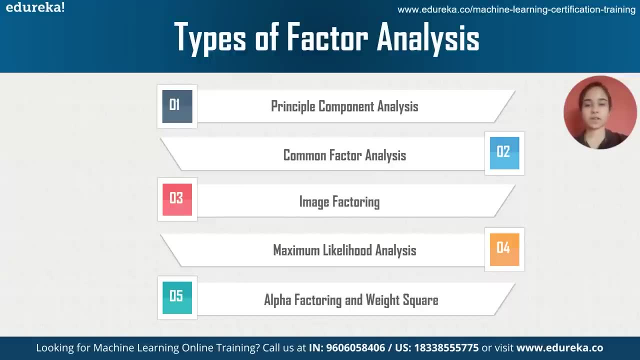 equations for modeling. the structure EFA is further divided into many types: The very popular PCA, or principal component analysis, common factor analysis or just factor analysis. image factoring that makes use of correlation matrix derived out of OLS regression maximum likelihood method. 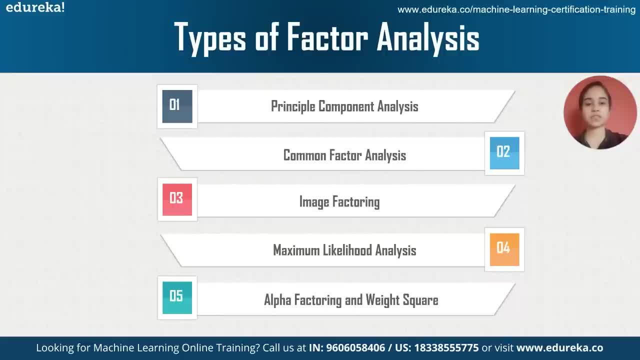 which is again based on the correlation matrix, and other methods such as alpha and beta Factoring and weight squared Out. of these, the most commonly used ones are principal component analysis and common factor analysis. Now let's go through some of the issues that we need to. 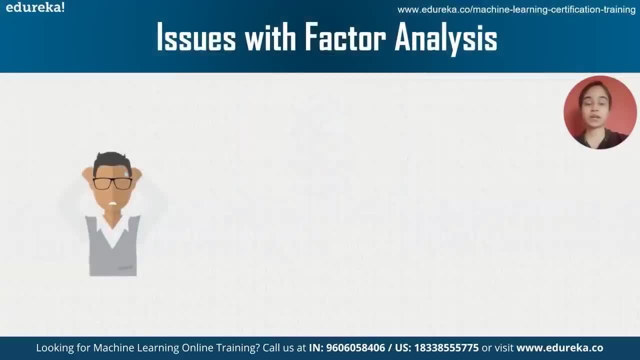 address with factor analysis. First, you need to understand whether to use principal component analysis or factor analysis. Next, you should know how to interpret the results of your analysis And finally, you need to figure out how many factors to pick. Let's address these issues one by one. 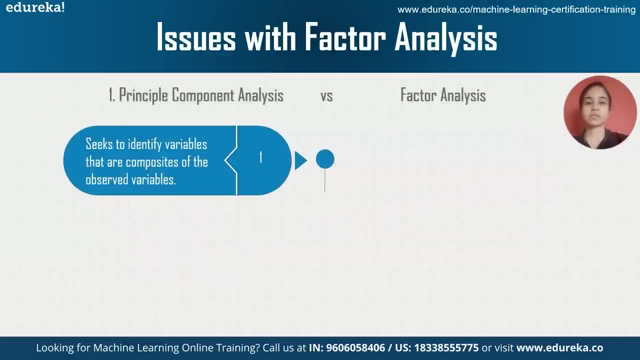 Principal component analysis tries to find the variables that are composites of observed variables, Such as in the house pricing dataset. PCA would identify that air quality index is closely determined by the number of parks in the locality. But in factor analysis we assume that 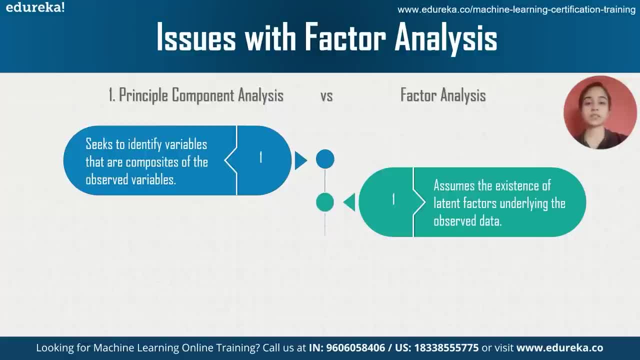 there are some latent factors, some immeasurable factors which can only be derived out of the given numeric variables. And secondly, in case of PCA, we take into account the total variance in the data, that is, the sum of unique variance, variance due to error and common variance. 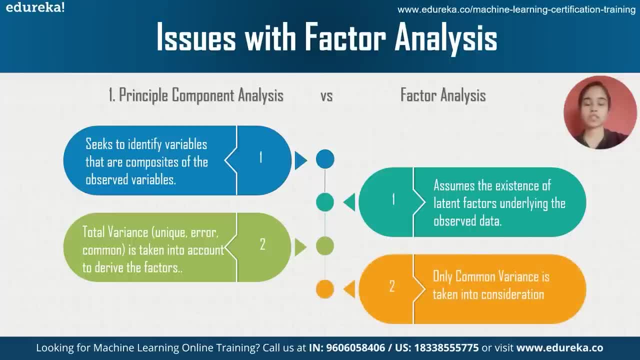 However, in factor analysis only the common variance of shared variance is considered. So when you want to find the latent variable using many variables, use factor analysis, and when you want to eliminate some variable that are having high variance, use PCA. When 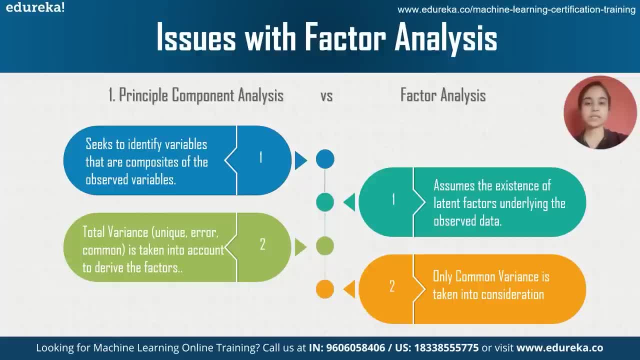 the number of variables is more than 30, the result of PCA and FA is the same. Next, you need to address how to interpret your stakeholders, like amount of variables, being Х in pause for a period of time. When your say F and Fälle, factor A, Q is what will be applied and HIV will be the same. 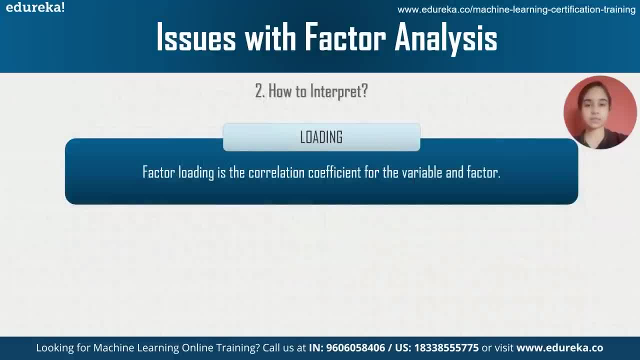 Next you need to address how to interpret the results of product analysis in general analysisnow the results of the analysis. For this we use something called loading. Factor loading is basically the correlation coefficient for the variable and factor. Factor loading shows the variance explained by the variable on that particular factor. Let's say you have 10. 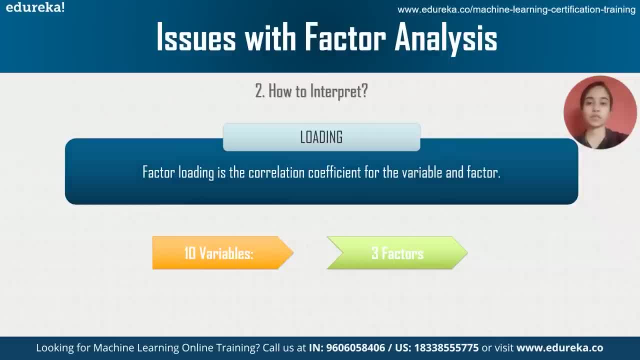 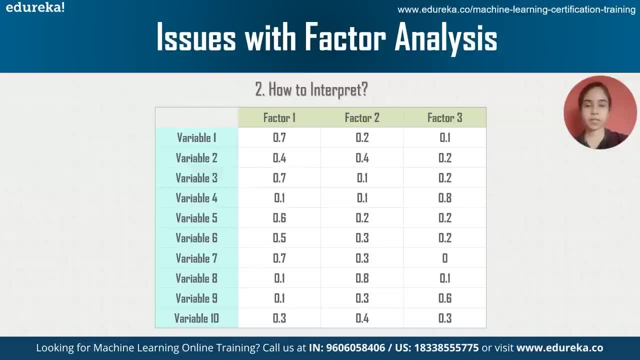 variables that you want to derive into three factors. So for that you make a table to account for how much of the variance of the variable is explained by a factor. It ranges from 0 to 1.. So if significant amount of the correlation is explained by a factor, the variable can be. 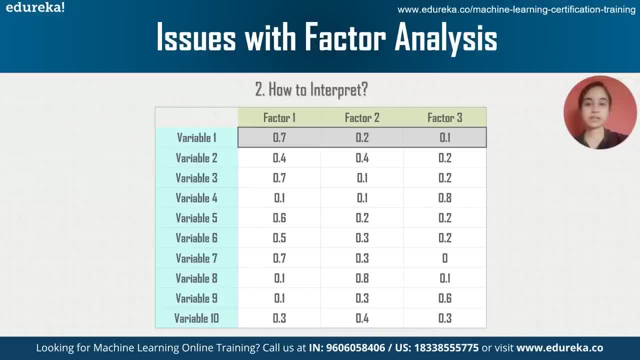 denoted. using that factor For deeper analysis, you can calculate the communality of a variable. It is given by the horizontal sum of squares of the values. For example, for variable 1, it would be 0.7 square plus 0.2 square plus 0.1 square. Similarly, the vertical sum of squares. 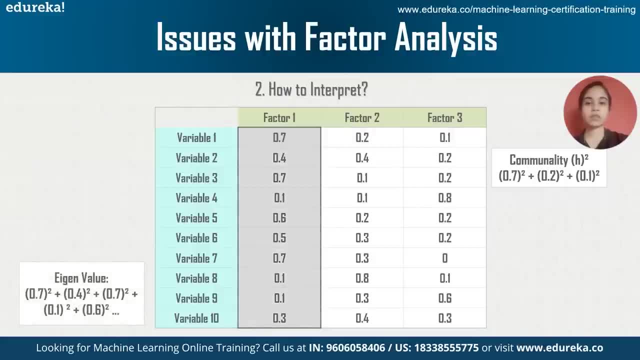 of values for a factor is called eigenvalue. For example, for factor 1, eigenvalue will be 0.7 square plus 0.4 square plus 0.7 square plus 0.1 square, and so on. Also sometimes for a particular variable. it shows high correlation. for more: 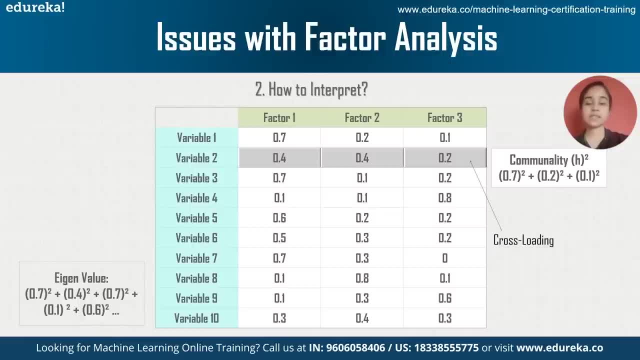 than one factor. This is called cross-loading, and in this scenario variable rotation should be performed. So we know how to interpret the results of the analysis. Now, how do we know how many factors to select When we talk about the sample? 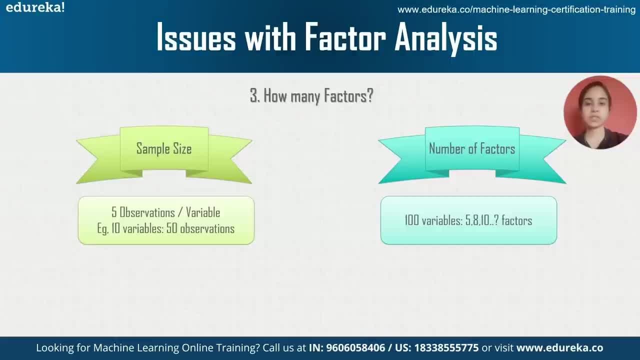 size. the rule of thumb is to have minimum 5 observations per variable. That is, for, let's say, 5 variables, you should have 25 observations, 10 variables, 50 observations and so on. But when it comes to deriving the factors of the variables, let's say, from 100 variables- 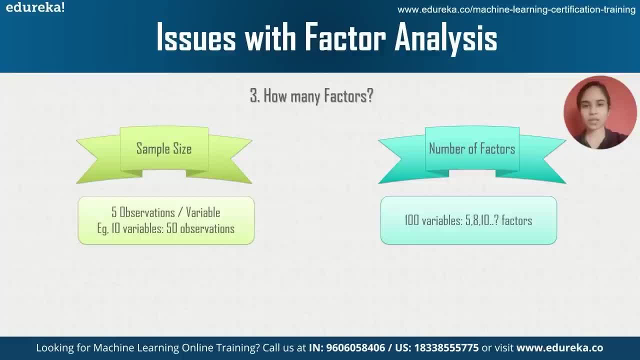 how do we know how many factors to take? 5,, 8,, 10, how many? For this you can make a scree plot and notice the bend in plot. However, this is not very intuitive. You can instead use: 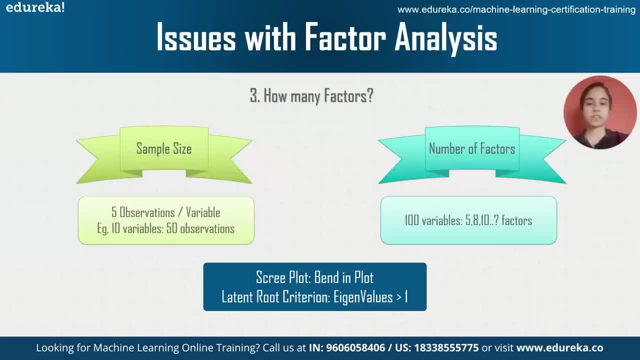 the substitute criterion, which states that, for a particular factor, if the vertical sum of squares of all the values, called the eigenvalue, is greater than 1, you should include that factor in your analysis. With that now, finally, let's go through the basic. 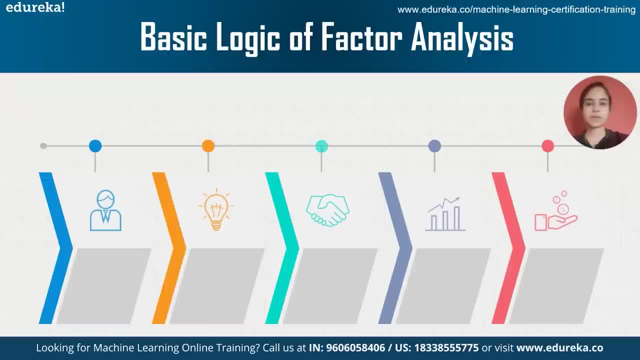 logic of factor analysis. Factor analysis basically gives you the items that you want to reduce. It creates a mathematical combination of variables that maximizes variance that you can predict in all variables, which is the principal component order and so on. New combination of items from recitable variance that maximizes variance you can predict. 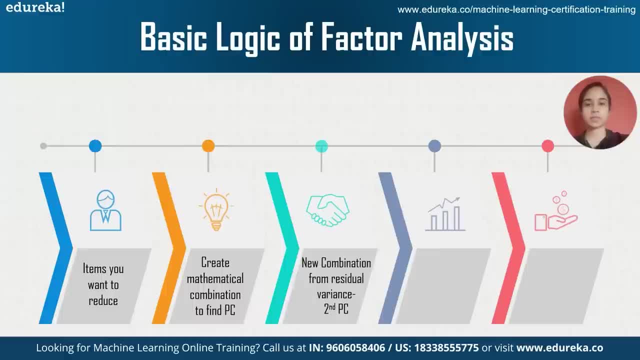 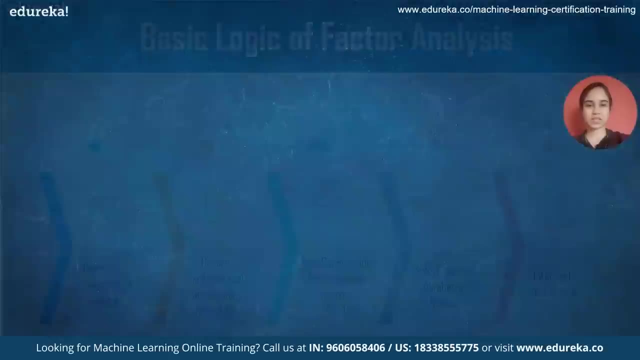 in. what is left is your second component or factor. Continue this until all the variance is accounted for and then select the minimal number of factors. With that, you can finally interpret the factors using rotated matrix and loadings. I hope you enjoyed the session. Thank you for watching this video. 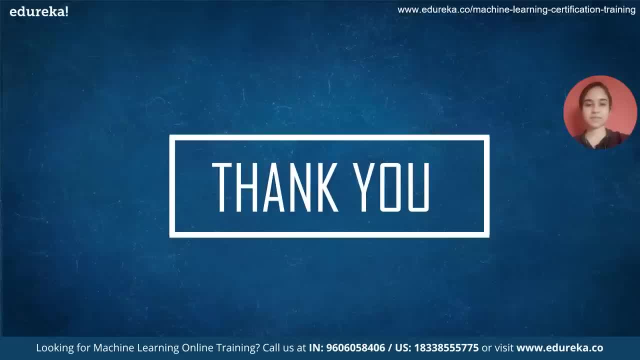 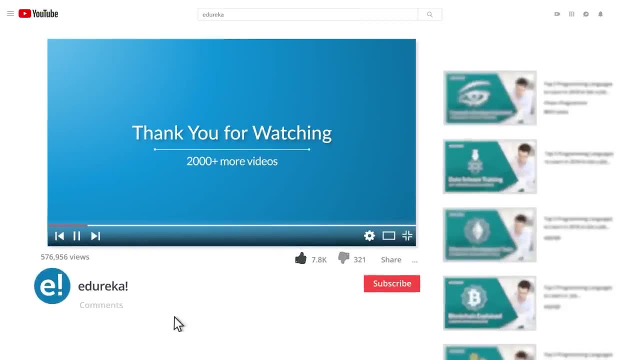 If you have any doubts, please leave a message in the comment section. Happy learning. I hope you have enjoyed listening to this video. Please be kind enough to like it and you can comment any of your doubts and queries and we will reply them at the earliest Do. 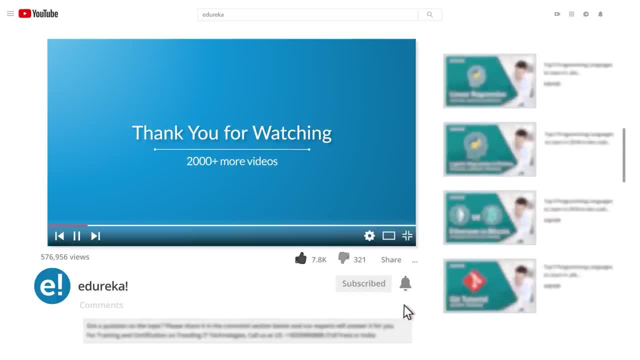 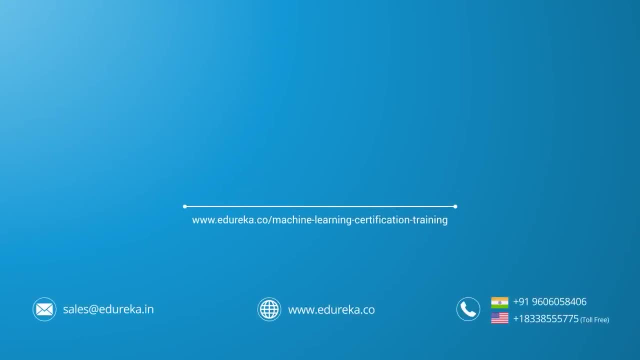 look out for more videos in our playlist and subscribe to Edureka channel to learn more Happy learning. Thank you for watching. 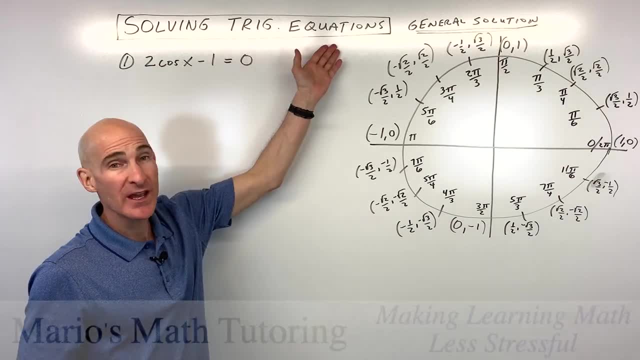 In this video you're going to learn how to solve trigonometric equations and, specifically, we're going to talk about how to find the general solution. So we're going to go through three examples, See if you can do these on your own, and we'll go through them together. The first one: 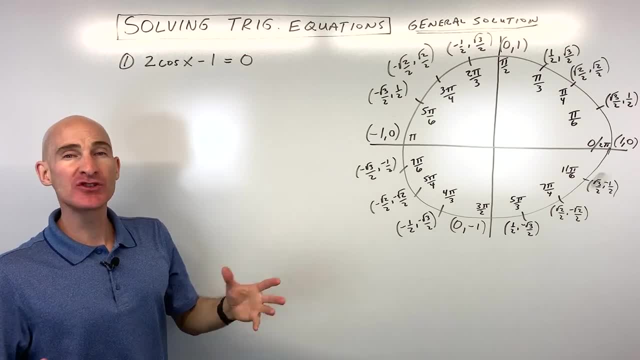 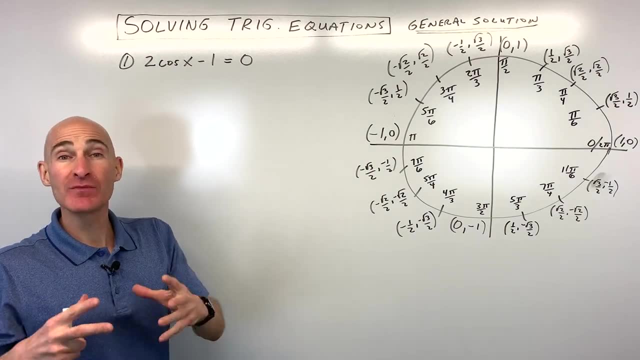 we've got two cosine x minus one equals zero. So when you're solving these trig equations, it's very similar to solving algebraic equations, but you want to get the trig function by itself on one side of the equation. So what we're going to do here is we're going to isolate this cosine of x. 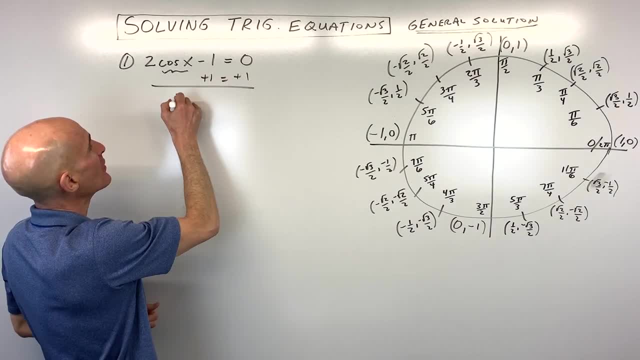 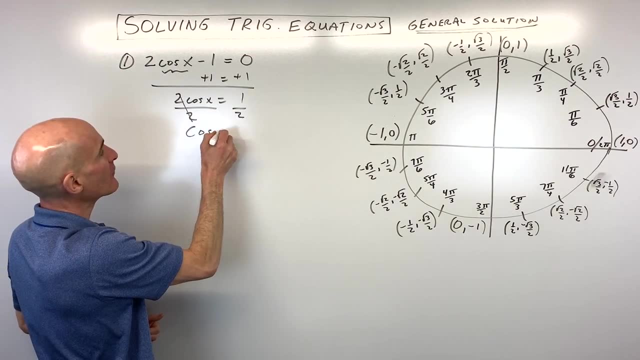 by adding one to both sides of the equation. so now we have two: cosine x equals one. We're going to divide both sides by two, and so now you can see that we have cosine of x equals one half. So now what we want to do is we want to go to the unit circle and want to ask ourselves: where is 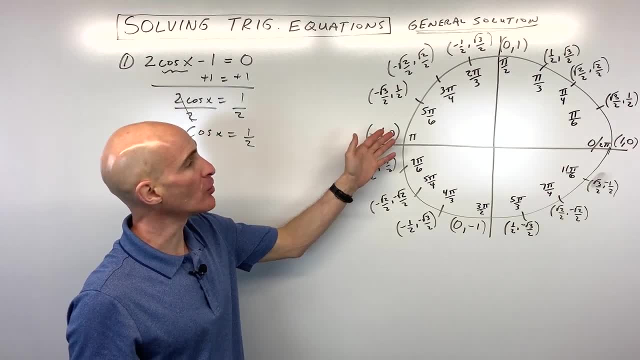 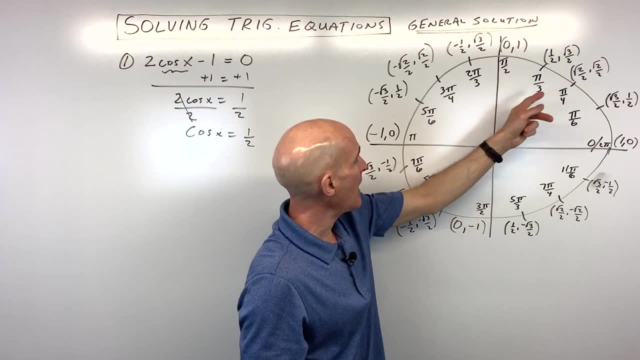 cosine equal to one half. well, remember, on the unit circle, cosine is the x coordinate, and so let's see where is the x coordinate of half? Well, we can see it's here as well as here. So if I just draw a little diagram, you can see that cosine is equal to one half, and what we're going to do is we're 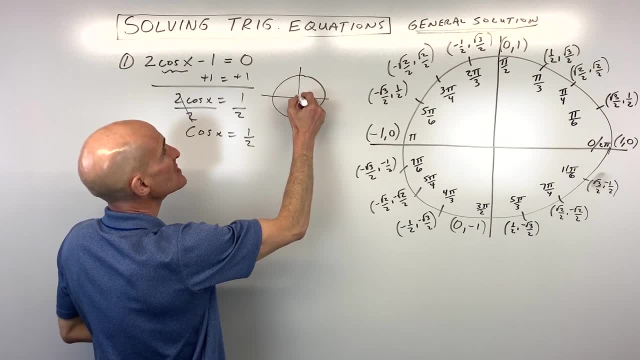 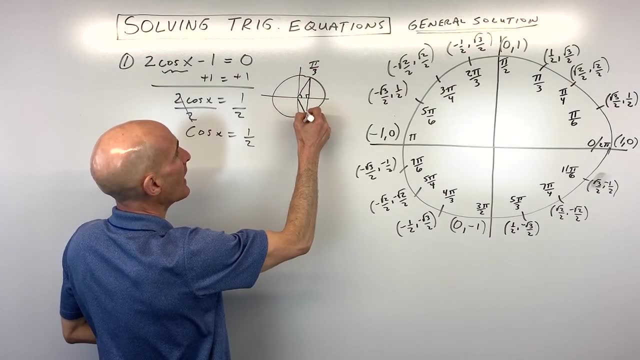 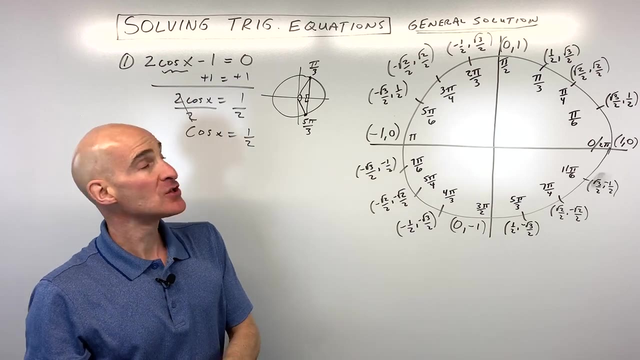 sketch over here just to illustrate. Here's our unit circle and you can see cosine's a half right here at pi over 3 or 60 degrees and over here at 5 pi over 3 or 300 degrees. Now notice these points here If we want to write a general. 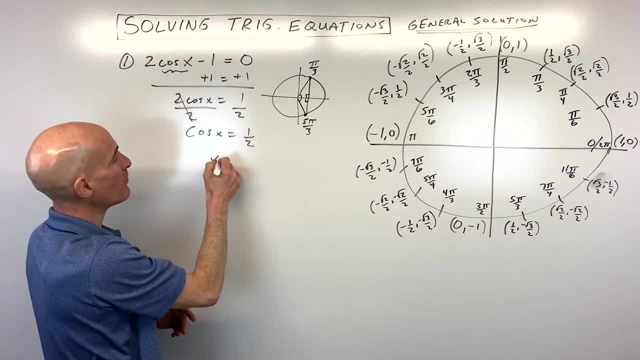 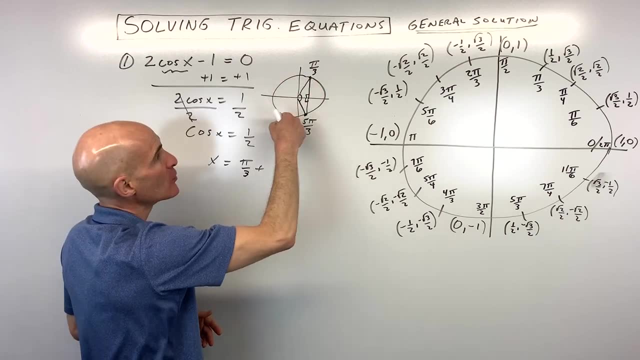 solution. what we have to do is we have to say x could equal pi over 3 plus if we add 2 pi or multiples of 2 pi, we're going to be going around that unit circle and we're going to be ending up in the same spot on the unit circle and